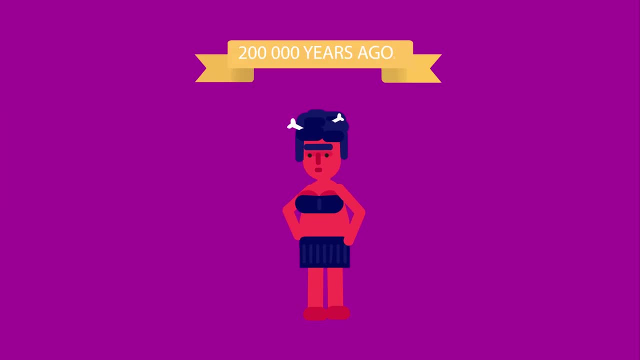 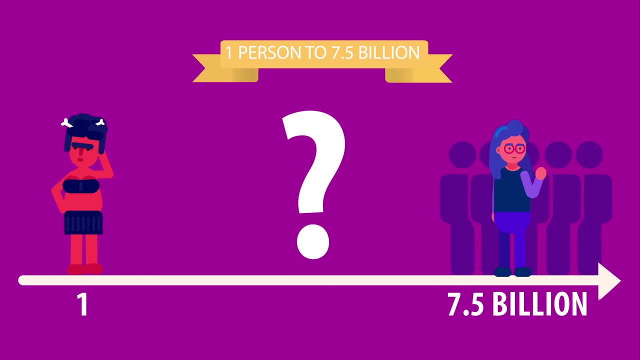 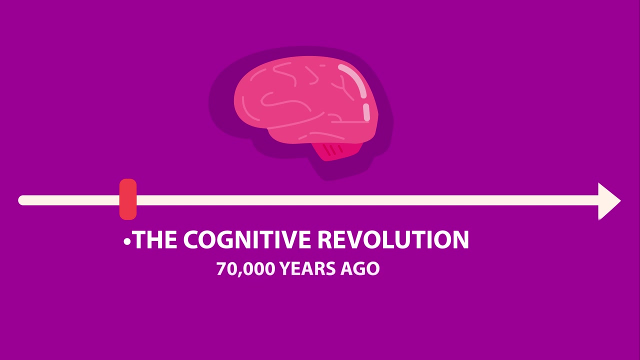 were extinct. During the past 200,000 years, we've grown from one person to the 7.5 billion today. What has that population growth been like? There have been 3 key revolutions: The cognitive revolution about 70,000 years ago, the agricultural revolution 12,000 years ago and the scientific. 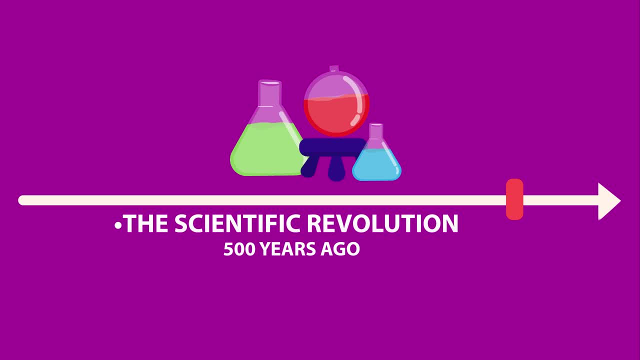 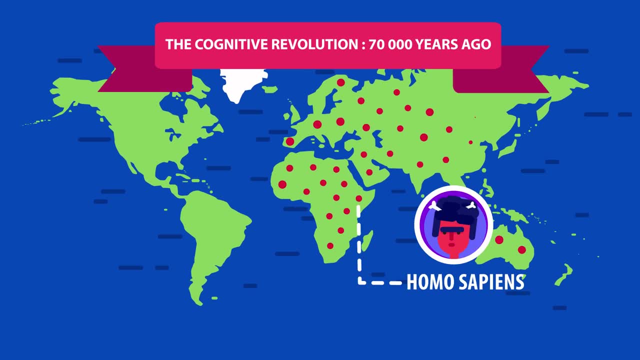 revolution of the past 500 years. all have been key players in global population. Homo sapiens population started the boom about 70,000 years ago, driving the other human species to extinction. Our ancestors conquered all corners of the earth and started inventing impressive objects. 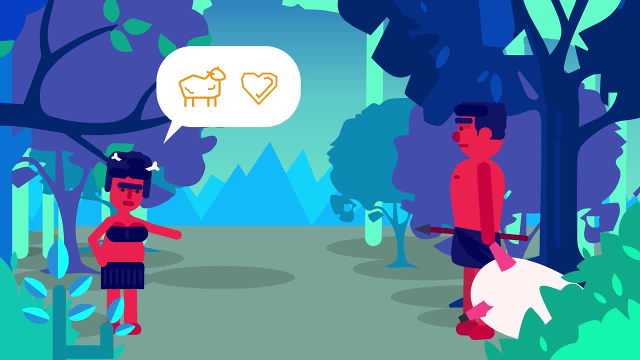 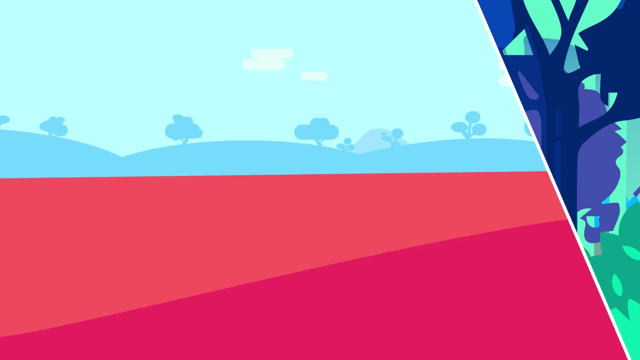 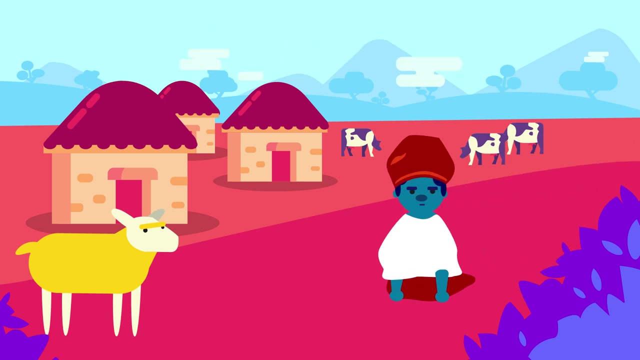 The most widely accepted explanation for our ancestors' rapid success is a huge improvement in our language abilities and therefore communication and ability to share information. 12,000 years ago, at the dawn of agriculture, there were about 5 million people alive. 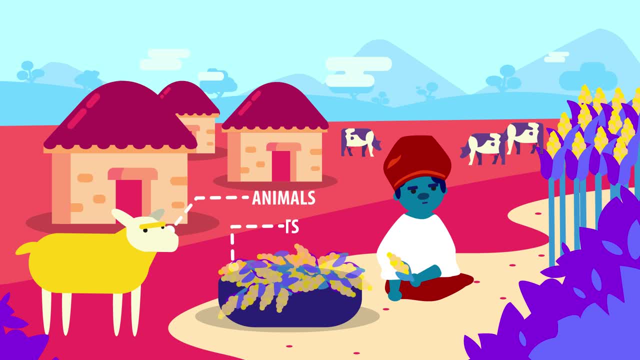 Our ancestors started farming some plant and animal species to provide them with a reliable supply of energy. 5 million people died in radius less than 500 years ago. We're growing Gay between 2 and 5 thousand. That's how that was. There's no nurse there in grenadeuckin'. 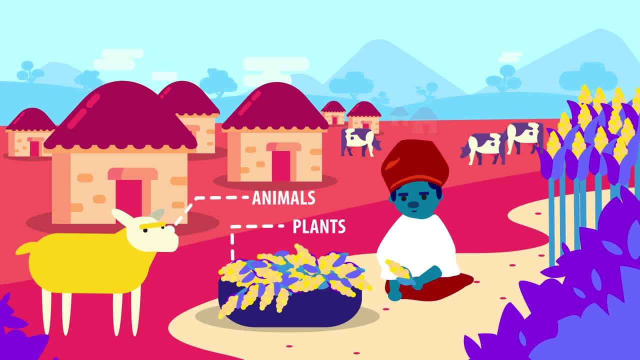 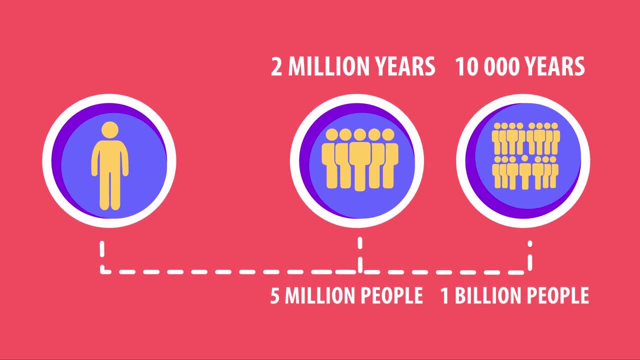 of energy, And this changed how we lived. People settled permanently around the fields and populations began to grow much more quickly than ever before. We took 2 million years to reach 5 million people, and then 10,000 years to reach 1 billion people, and that's. 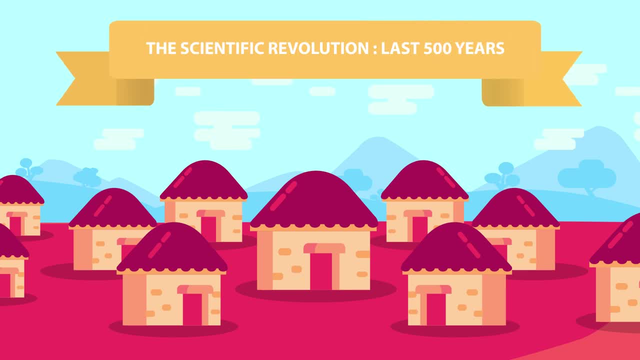 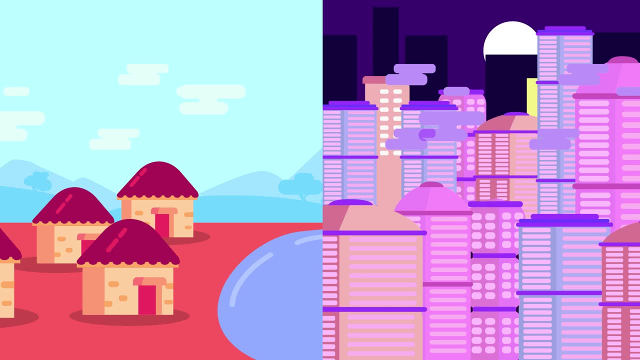 nothing compared to what was to come. Welcome to the science revolution. 200 years ago, the global population was about 1 billion people. Now we're at a huge 7.5 billion today, And still every year there are 83. 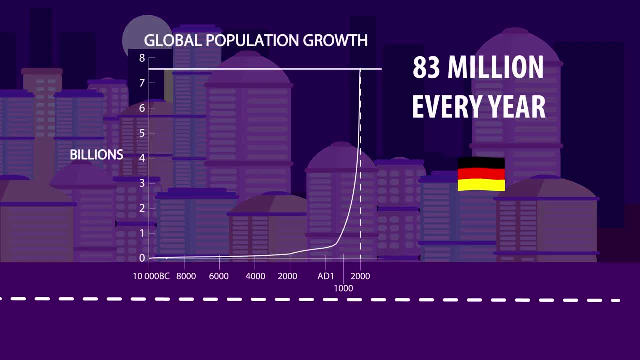 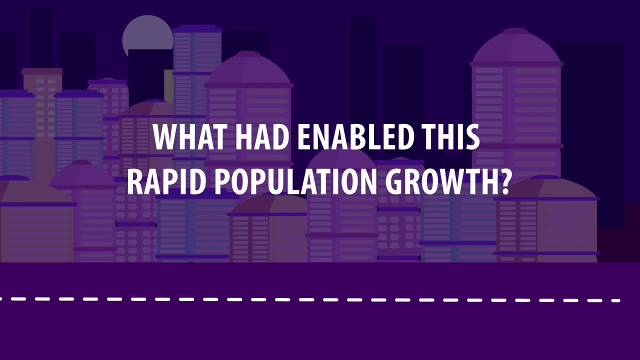 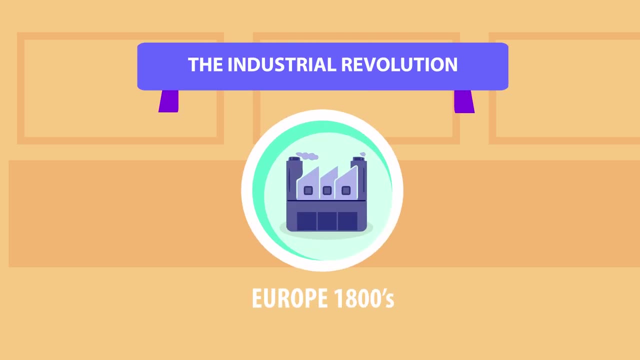 million more people living on this planet. That's the population of the entire of Germany. So what's happened in the last few hundred years to enable this rapid population growth? It started with a further agricultural revolution in Europe in the 1700s, and then the industrial 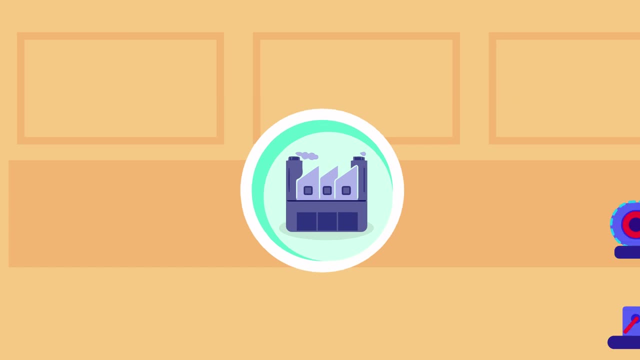 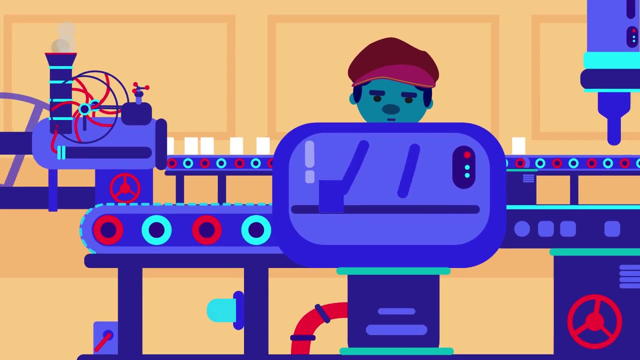 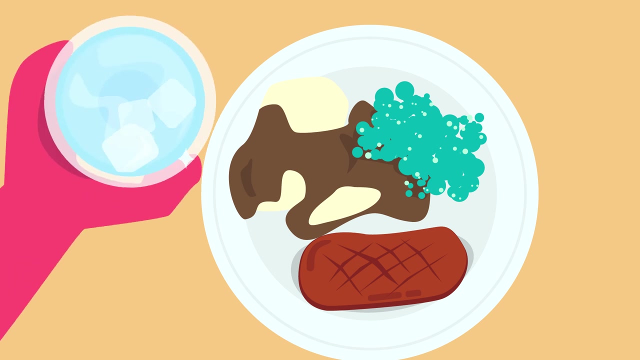 revolution of the 1800s, The invention of the steam engine. The steam engine increased food production, better employment rates and wages, improved quality of healthcare and standards of living have enabled a massive population boom. In simple terms, because there was more food and clean water to go around, less disease. 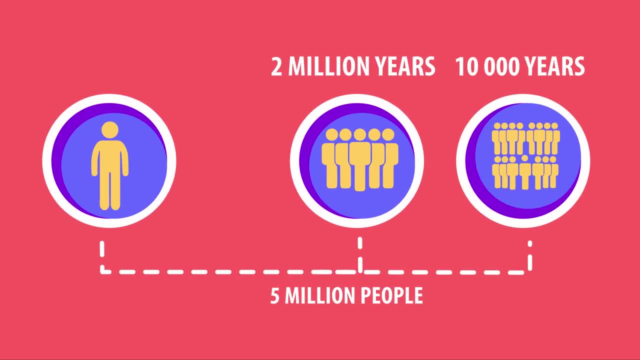 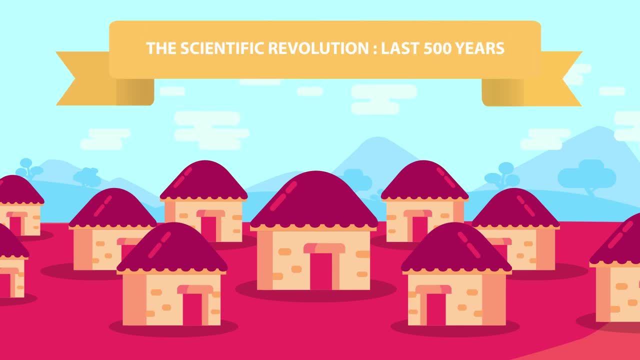 to reach 5 million people, and then 10,000 years to reach 1 billion people. and that's nothing compared to what was to come. Welcome to the science revolution. 200 years ago, the global population was about 1 billion. 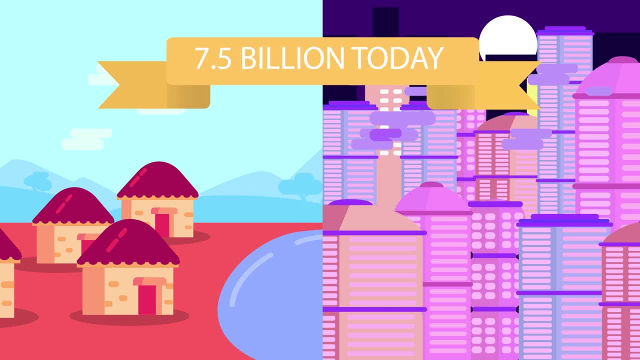 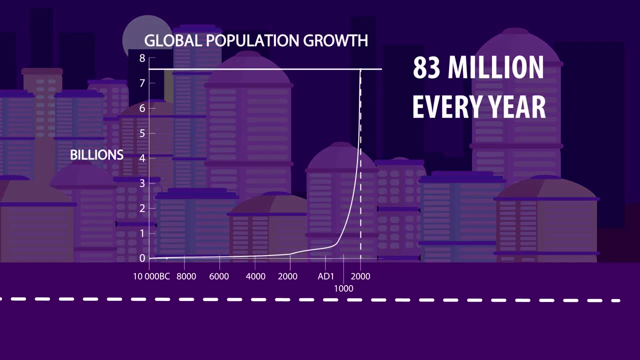 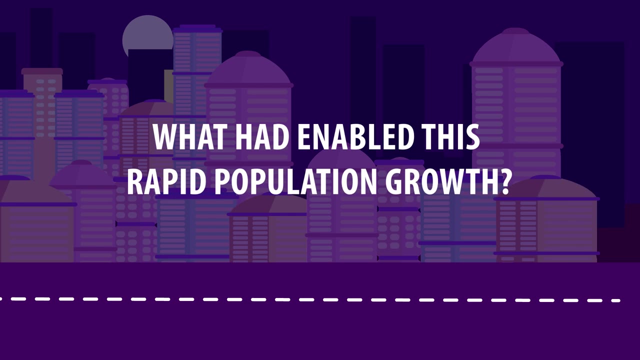 people. Now we're at a huge 7.5 billion today, And still every year there are 83 million more people living on this planet. That's the population of the entire of Germany. So what's happened in the last few hundred years to enable this rapid population growth? 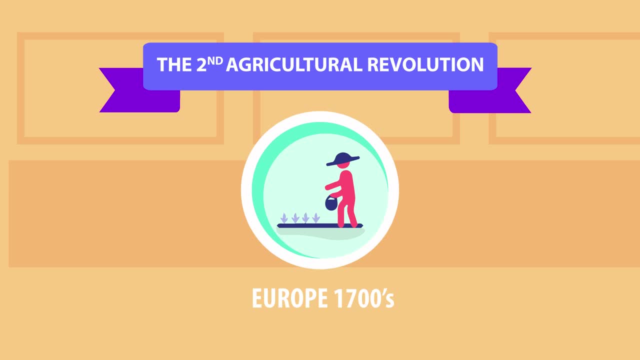 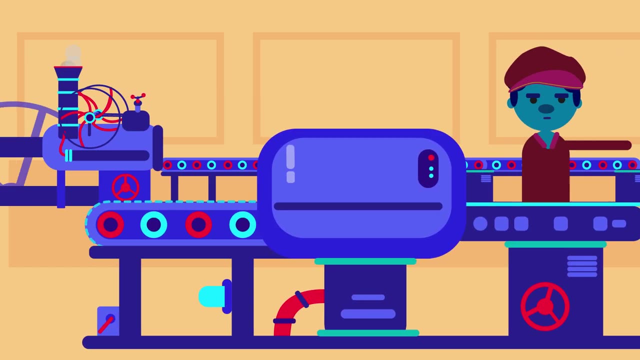 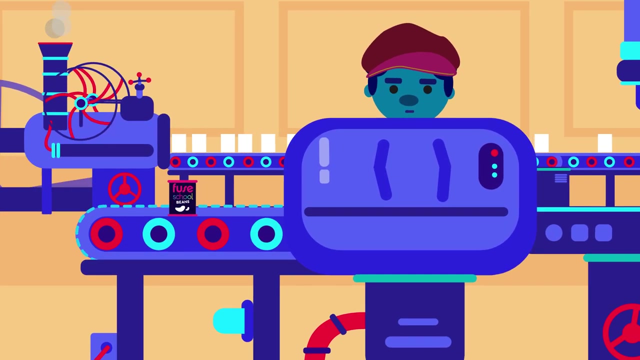 It started with a further agricultural revolution in Europe in the 1700s and then the industrial revolution of the 1800s, The invention of the steam engine. The steam engine, increased food production, better employment rates and wages, improved quality of healthcare and standards of living- have enabled a massive population boom In. simple terms, because there was more food and clean water to go around, less disease and better medical care for the sick. it meant fewer people died. People that would otherwise have died survived, increasing the population. They then had children themselves, further increasing the population, and so the story goes on. 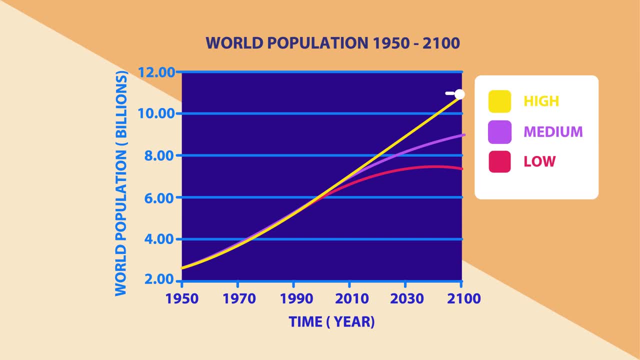 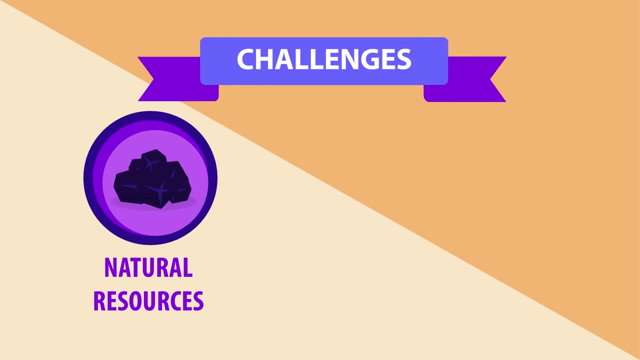 So what next? We're expected to be over 11 billion by the year 2100. But the truth is, nobody is certain To support the growing population. the world's economy is expected to triple in size in this century alone. All of this is a massive challenge for the Earth's. 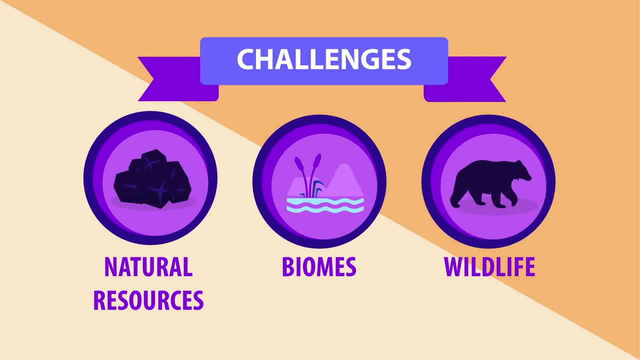 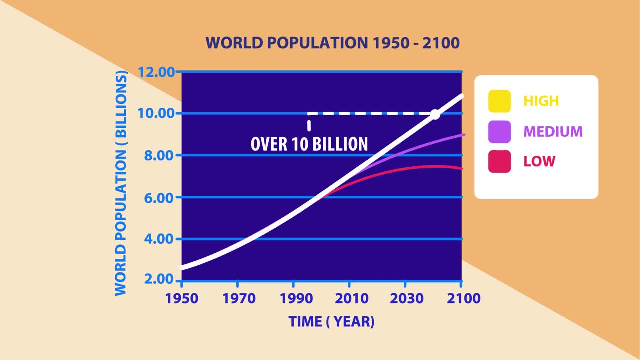 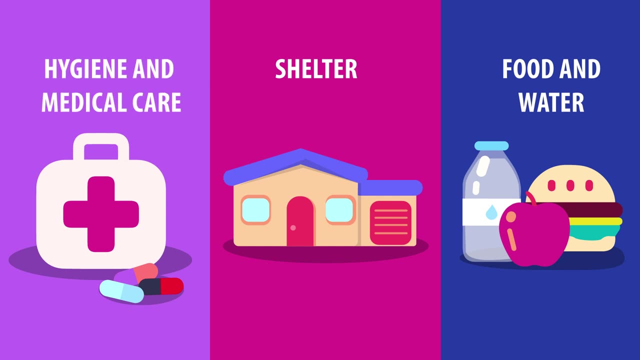 natural resources, biomes and wildlife. Population could continue to grow at its current rate, creating a world population of over 10 billion in the next 30 years. For this to happen, there needs to be enough food, water, shelter, and the hygiene and medical care is good. 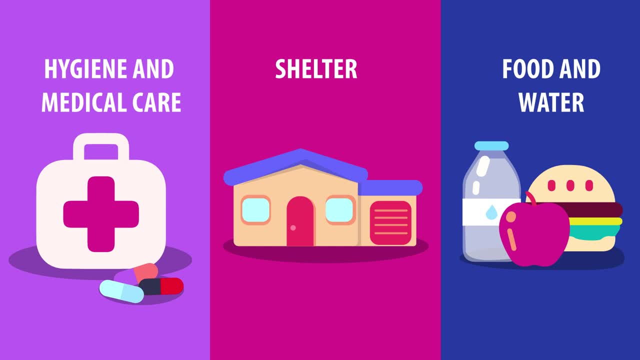 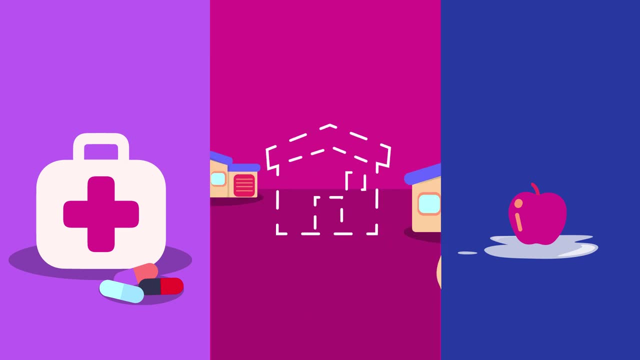 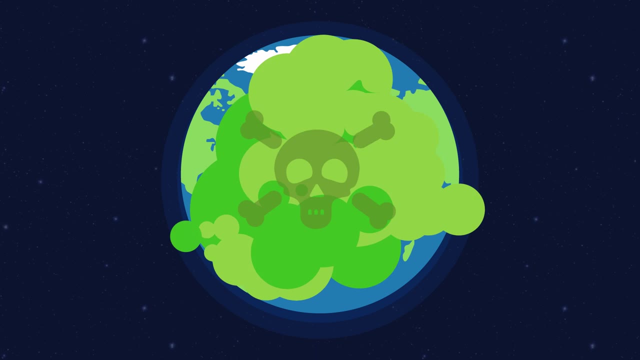 Or maybe global population decreases. There might be insufficient resources to share. Maybe food and water become scarce Or not enough housing for everyone, Or medical care that prevents diseases and saves lives may not be available to everyone. Maybe our irresponsible use of antibiotics today could result in a global epidemic in the near future. 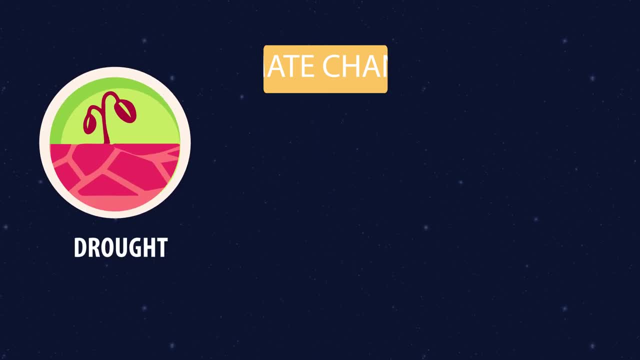 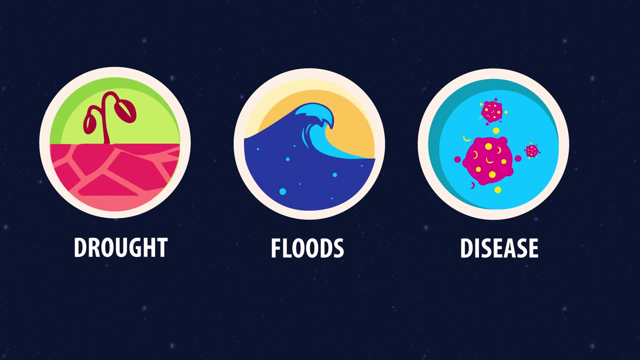 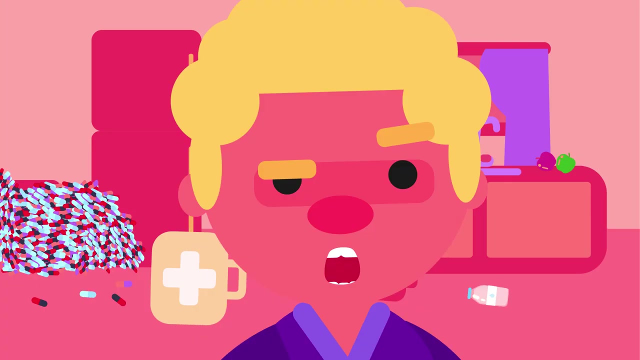 Or our human-induced climate change could result in serious drought or damaging floods, thus bringing famine or disease with it. So this all sounds rather scary. considering 2050 will probably be in most of your lifetimes. Before you start panicking and stockpiling food and medicines like you're in a zombie movie, remember, even the experts aren't sure. 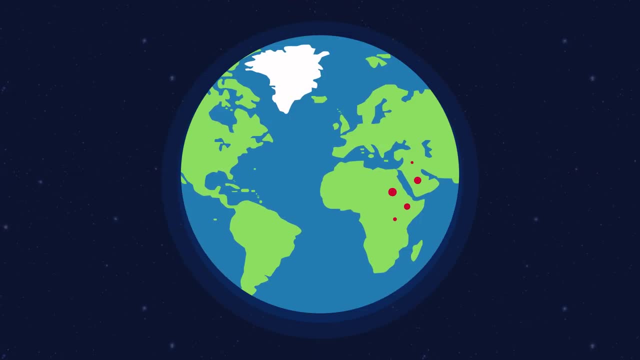 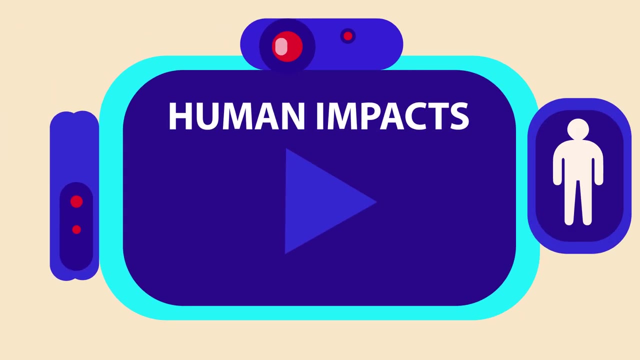 We just don't know what's going to happen. All we do know is the Earth's population will change over the coming decades. To learn about the impacts of climate change, visit wwwnasagovau. To learn about the impacts of humans on our planet and how we can develop and grow in a sustainable way. watch these videos. 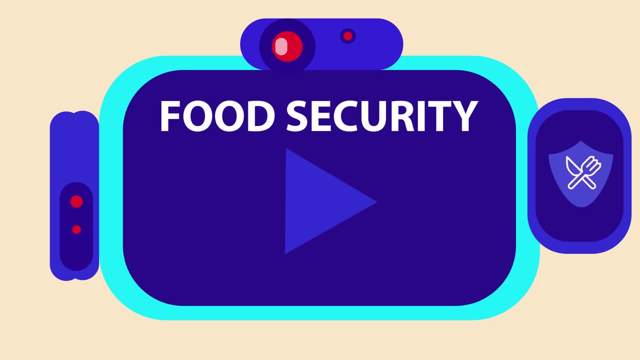 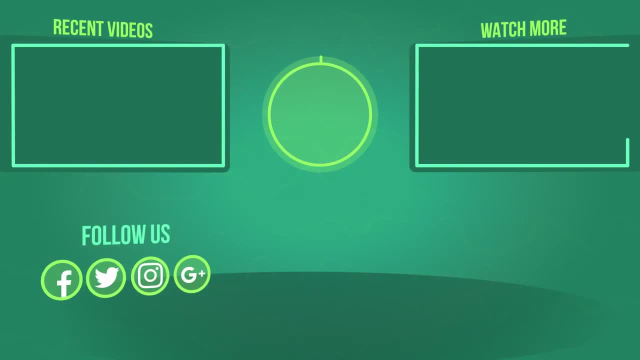 And with a growing population. food security is, and will continue to be, an important issue which we investigate further in this video. If you liked the video, give it a thumbs up And don't forget to subscribe. Comment below if you have any questions. Why not check out our Fuse School app as well? Until next time. 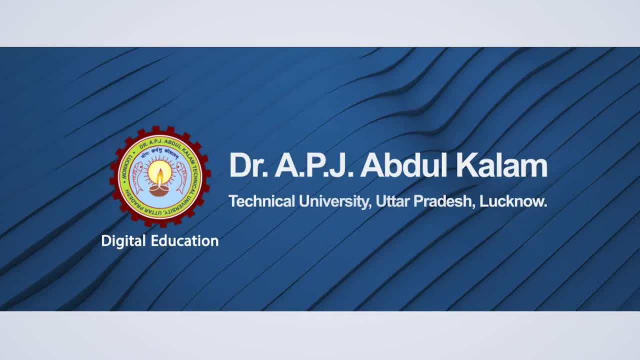 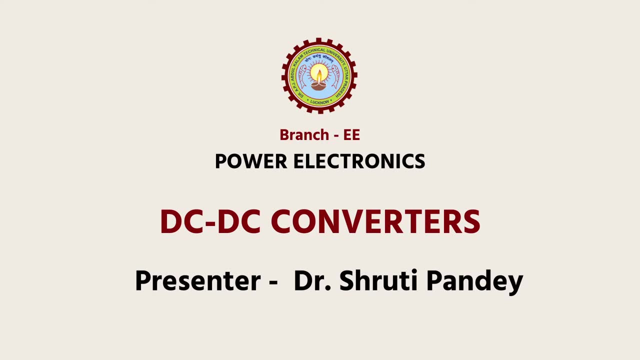 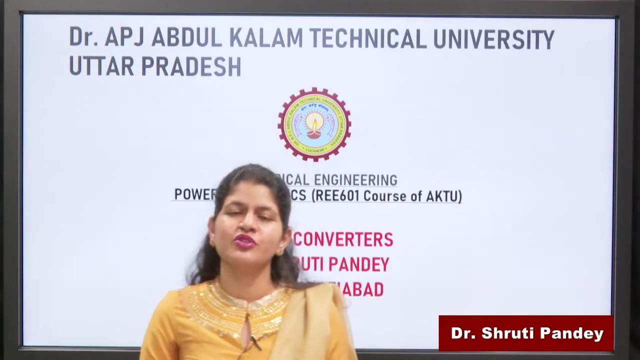 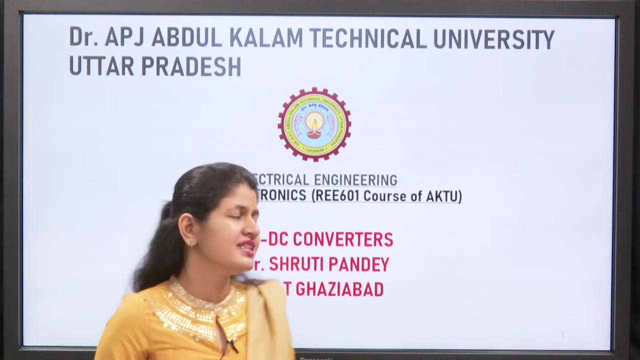 Hello everyone, I am Dr Shruti Pandey. I am working as an assistant professor at Kite Group of Institutions and today the topic I will be dealing with is DC to DC converters. DC to DC converters is one of the most widely used and one of the most versatile power converters. 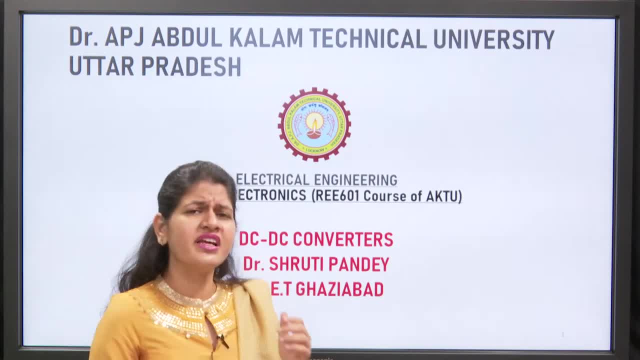 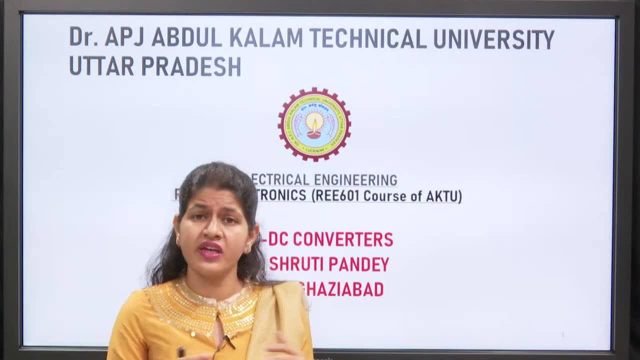 in whole power electronics engineering. They are not only important from gate point of view or your end semester point of view or engineering services point of view. it is also very important as we deal with industrial applications. Industrial applications, say. what I mean is renewable energy industry and all the renewable energy resources, whether you take PV resource. 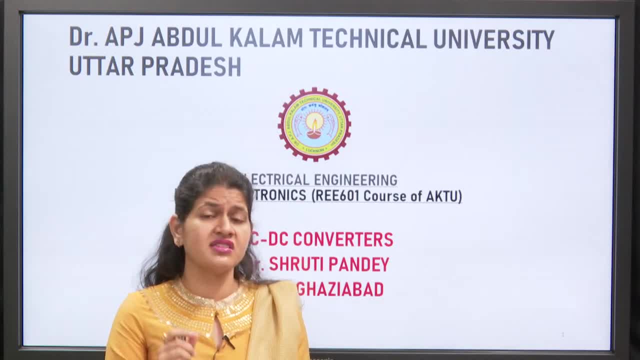 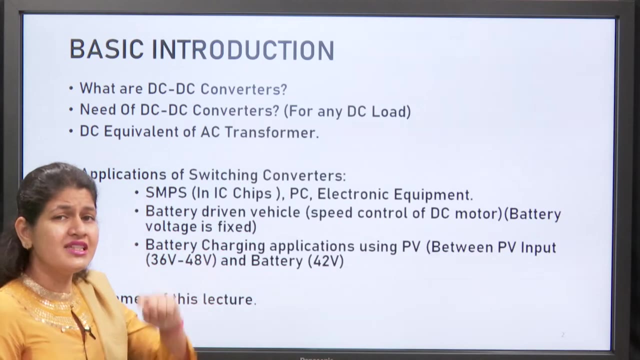 or wind resource, any resource. DC to DC converters are most widely used and they are very much helpful in obtaining the desired as well as most efficient output. So we will move towards the first slide. First is basic introduction. First, what are DC to DC converters? So DC? 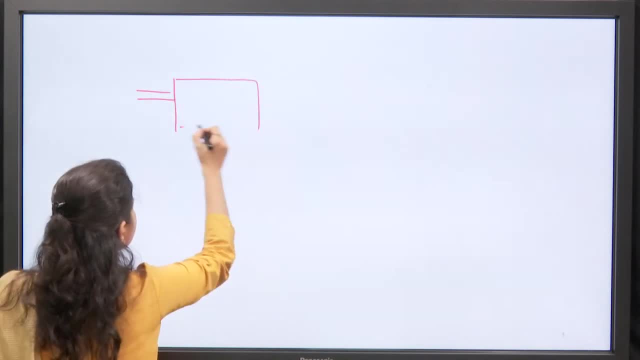 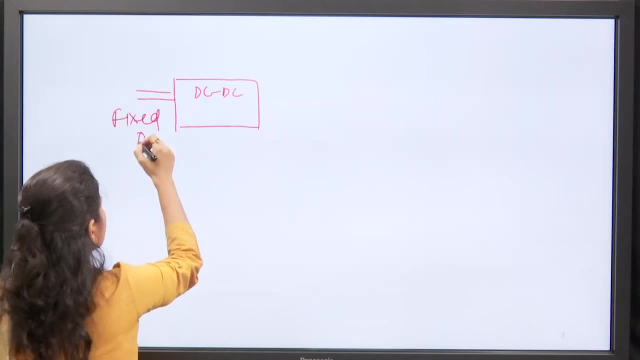 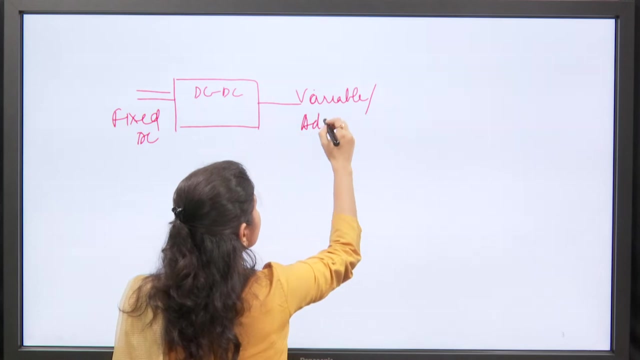 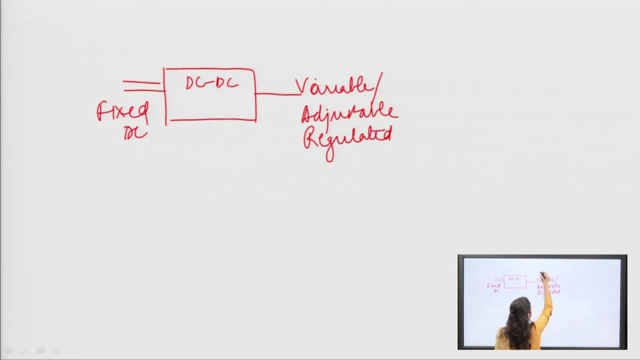 to DC converters are basically DC to DC converters are basically those converters which converts fixed DC to Variable DC. And by variable, what do I mean? washable, adjustable, or regulated or controlled? Ok, Suppose that there is an application, the power supplies. 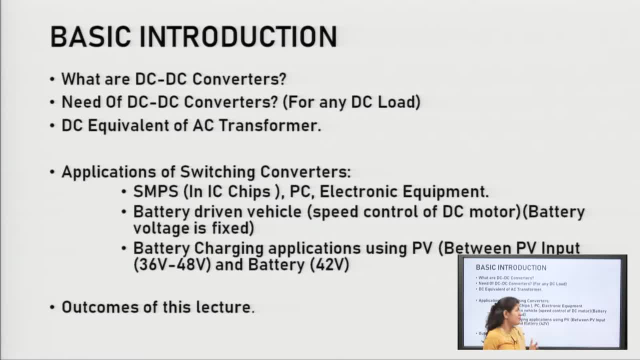 available in our labs. suppose they are 12 volts. Ok, So 12 volt DC power supply we get in labs and we can over here, how many power supplies do we get? So we just think that 12 volts are very less than 12 volts necessary for a charger If we subtract 12.